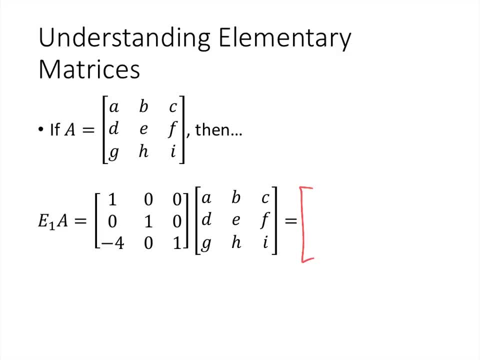 first row and down each of the columns. what we're just gonna get is A, B, C. So we multiply 1 by A, 0 by D, 0 by G. Add those results together, we just get A. Similarly, 1 times B, 0 times E, 0 times H. Add those together, we get B Similarly. 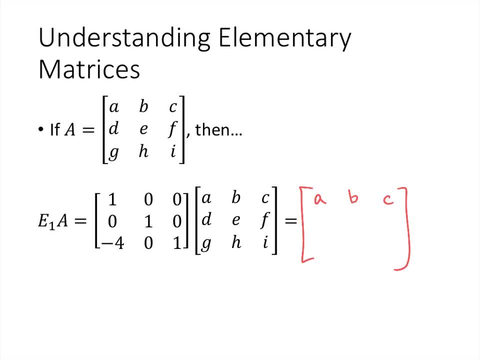 when we go down the second row, across the second row of the matrix E1, and down the columns of the matrix A, we just get D, E, F. But now something different is gonna happen when we go across the third row of matrix E1.. We're gonna get 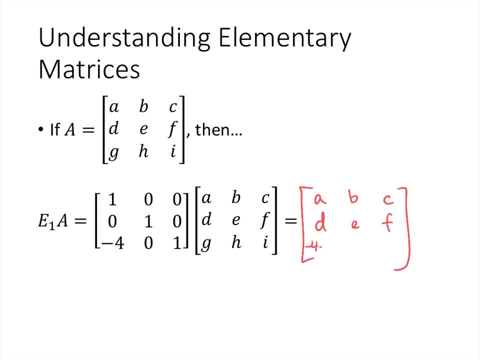 negative 4 times A plus G, We're gonna get negative 4 times B plus H, And we're gonna get negative 4 times C plus I. And so notice that the result of multiplying E1 by A is that we did the same row operation. 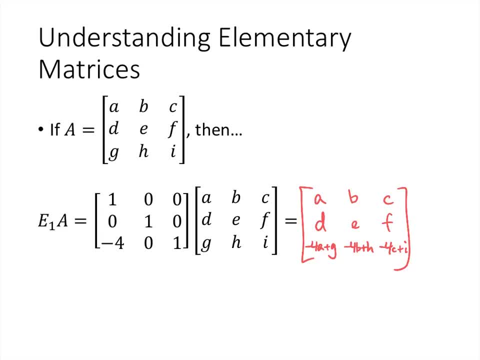 that we were talking about, but we did it to the matrix A. In other words, we replaced row 3 by negative, 4 times row 1 plus row 3.. That's the result of what has happened. We replaced row 3 by negative 4 times row 1 plus row 3.. We did that same replacement. 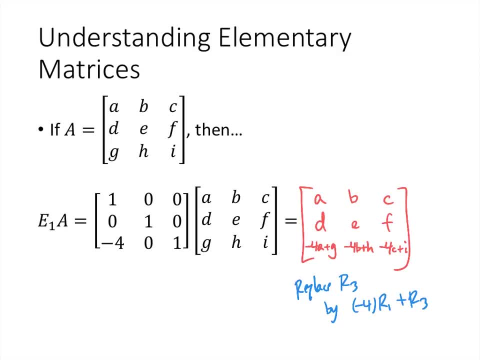 operation that created the matrix E1,, but we've done it to A rather than doing it to D. We did that same replacement operation that created the matrix E1,, but we've done it to A rather than doing it to D. We did that same replacement operation that created the matrix E1,, but we've done it to A rather than doing it to D. 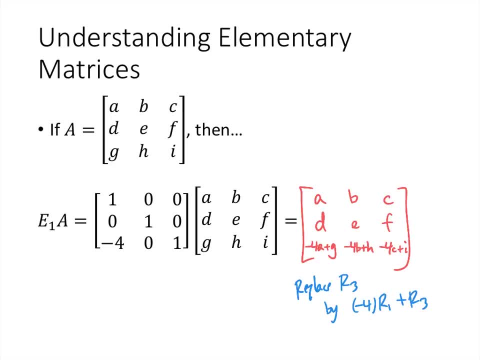 And the same would be true about the matrices E2 and E3 that we talked about. Multiplying a matrix by an elementary matrix gives you, as a result, what you would get if you did that elementary row operation to that matrix that you multiply by. So let's see that here, When we multiply by E2, the result that 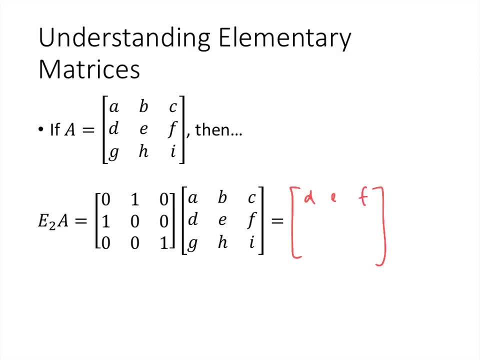 we're going to get is D, E, F in the first row, A, B, C in the second row and G, H, I in the third row. So the result is that we've swapped rows 1 and row 2 of A by multiplying E2 by A. Similarly, when we multiply E3 by A, the result is going: 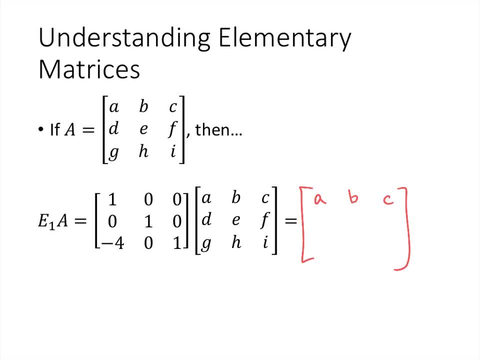 when we go down the second row, across the second row of the matrix E1, and down the columns of the matrix A, we just get D, E, F. But now something different is gonna happen when we go across the third row of matrix E1.. We're gonna get 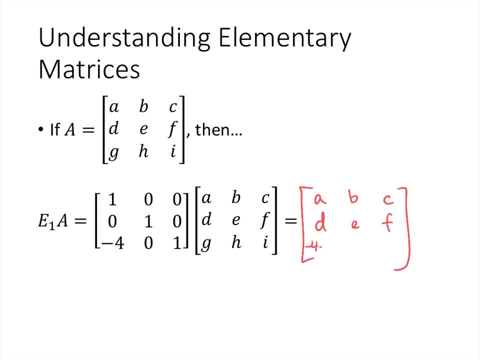 negative 4 times A plus G, We're gonna get negative 4 times B plus H, And we're gonna get negative 4 times C plus I. And so notice that the result of multiplying E1 by A is that we did the same row operation. 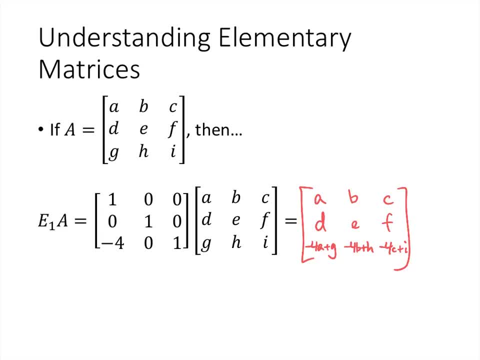 that we were talking about, but we did it to the matrix A. In other words, we replaced row 3 by negative, 4 times row 1 plus row 3.. That's the result of what has happened. We replaced row 3 by negative 4 times row 1 plus row 3.. We did that same replacement. 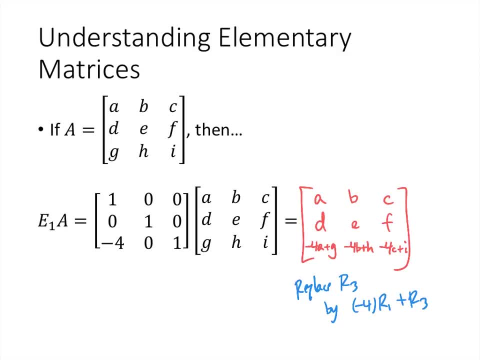 operation that created the matrix E1,, but we've done it to A rather than doing it to D. We did that same replacement operation that created the matrix E1,, but we've done it to A rather than doing it to D. We did that same replacement operation that created the matrix E1,, but we've done it to A rather than doing it to D. 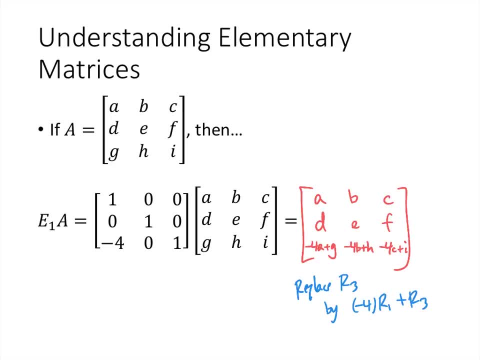 And the same would be true about the matrices E2 and E3 that we talked about. Multiplying a matrix by an elementary matrix gives you, as a result, what you would get if you did that elementary row operation to that matrix that you multiply by. So let's see that here, When we multiply by E2, the result that 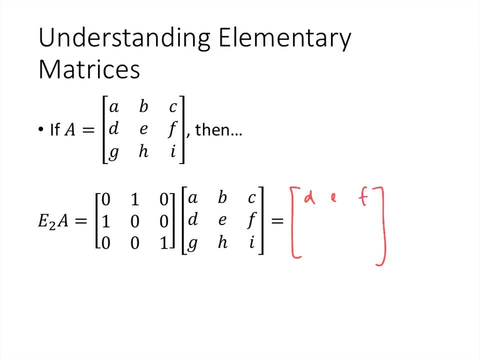 we're going to get is D, E, F in the first row, A, B, C in the second row and G, H, I in the third row. So the result is that we've swapped rows 1 and row 2 of A by multiplying E2 by A. 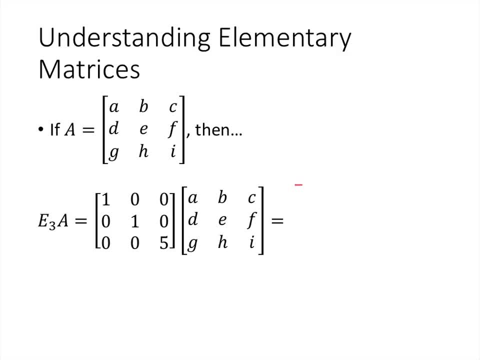 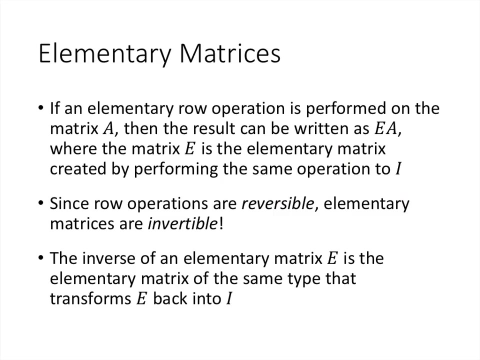 Similarly, when we multiply E3 by A, the result is going to be that we will scale row 3 by a factor of 5, bringing it 5G, 5H and 5I in that third row. So the conclusion here is that an elementary row operation, if we perform, 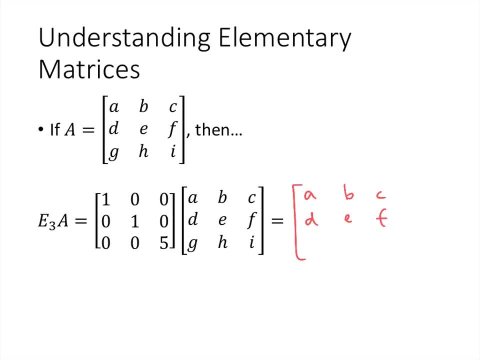 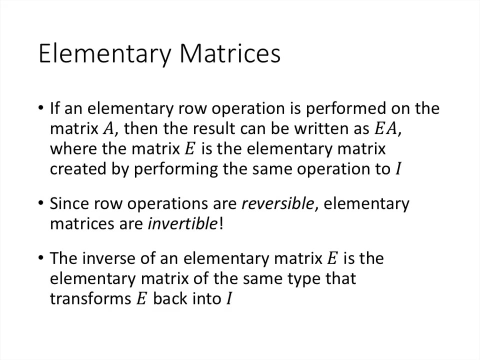 to be that we will scale row 3 by a factor of 5, bringing it 5G, 5H and 5I in that third row. So the conclusion here is that in the elementary row operation if we perform that on matrix A, then we can represent the result in a matrix multiplication. 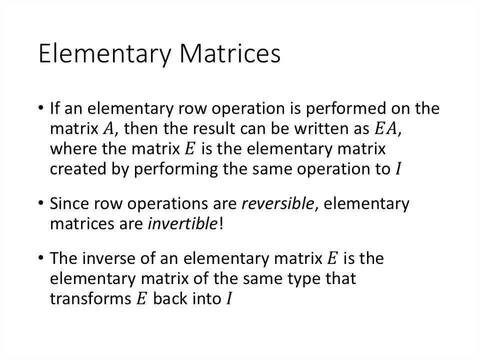 form We can represent the result of doing that row operation as E, where E is the elementary and matrix. An important observation here is that because row operations are reversible, elementary matrices have to be invertible, because all we do the inverse of an elementary matrix would just be to 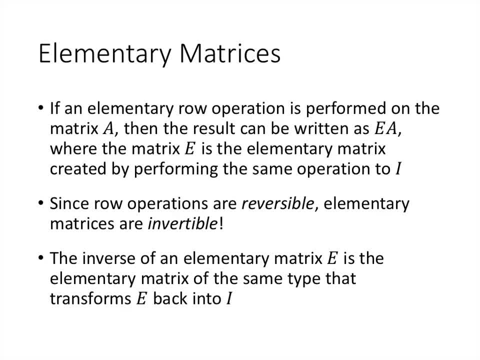 multiply by the opposite of that row operation. If you swap rows 1 and 2, then you just swap them back. If you added 4 times row 3 to row 2, you add negative 4 times row 3 to row 2.. If you scaled a row by a factor of 3, then you scale it again by a factor of 1- third. So all. 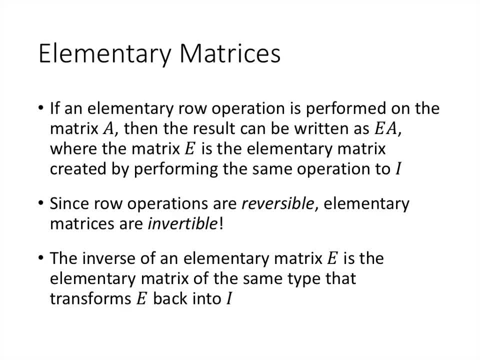 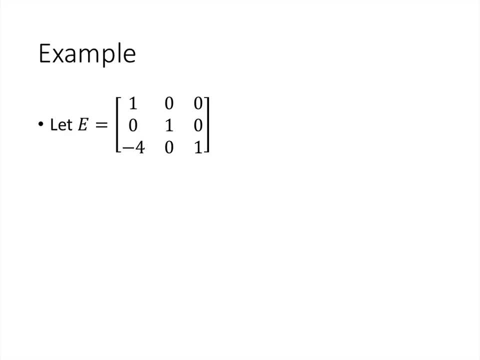 of those elementary matrices. those are all invertible matrices and we can tell exactly what the inverses would be. So in this case, if E is this elementary matrix that we got by replacing row 3 by negative, 4 times row 1 plus row 3, then the inverse, if we believe what we, 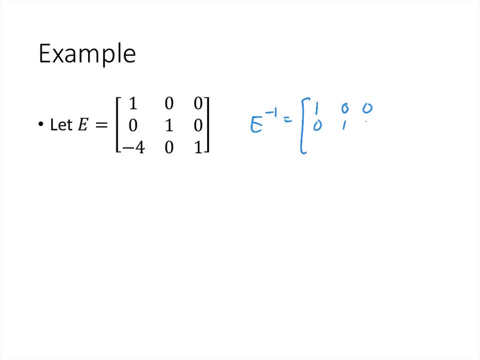 just said on the previous slide, would be the opposite row operation, which would be to replace row 3 by positive 4 times row 1 plus row 3.. And let's just check and make sure this works out. Remember to verify that two matrices are inverses. we multiply them in both possible orders. 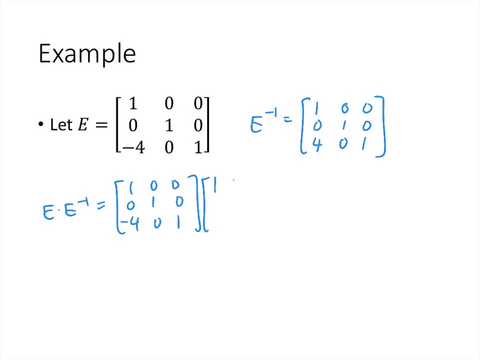 and make sure that we actually get the identity. And when we multiply this out, lo and behold, we do in fact get the identity matrix, with ones down the diagonal and zeros everywhere else. Similarly, when multiply in this order again, we get the identity matrix. 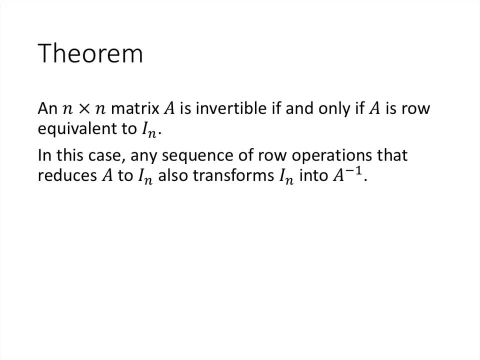 ok, so what are all these elementary matrices good for? Well, we have this theorem which is going to tell us exactly how to figure out, first of all, when a matrix is invertible and, in addition to that, how to actually figure out what the inverse of that matrix is. So the theorem says two things. It 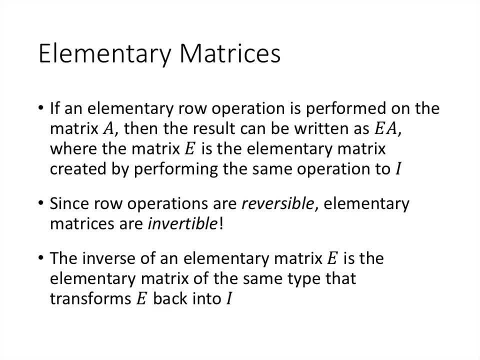 that on the matrix A. then we can represent the result in a matrix multiplication form. We can represent the result of doing that row operation as E A, where E is the elementary matrix. An important observation here is that because row operations are reversible, elementary matrices have to be: 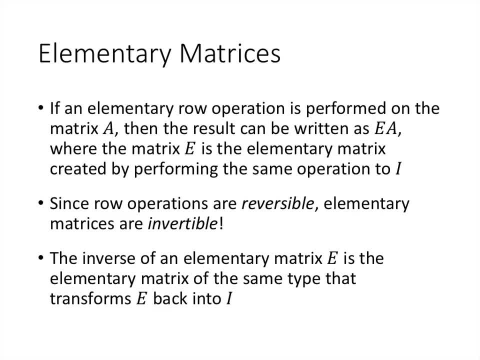 invertible, because all we do the inverse of an elementary matrix would just be to multiply by the opposite of that row operation. If you swapped rows 1 and 2, then you just swap them back. If you added 4 times row 3 to row 2, you add. 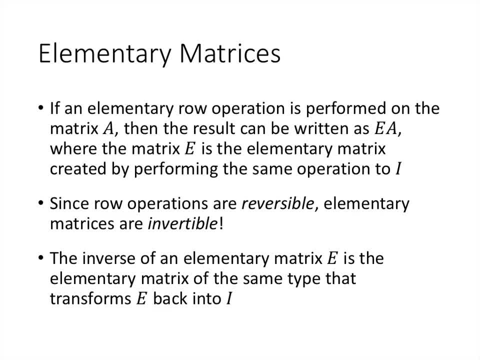 negative 4 times: row 3 to row 2. If you scaled a row by a factor of 3, then you scale it again by a factor of 1, 3rd. So all of those elementary matrices, those are all invertible matrices and we can tell exactly what the inverses would be. 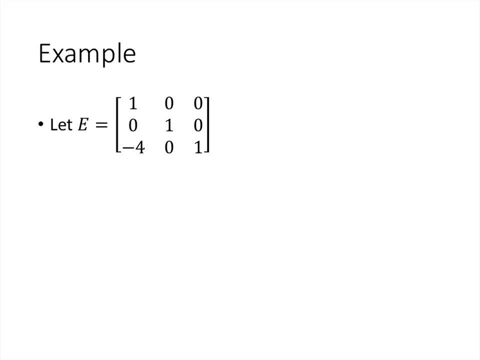 So, in this case, if E is this elementary matrix that we got by replacing row 3 by negative, 4 times row 1 plus row 3, then the inverse, if we believe what we just said on the previous slide, would be the opposite row operation, which would be to: 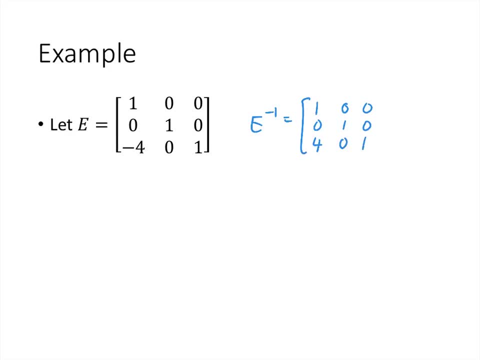 replace row 3 by positive, 4 times row 1 plus row 3.. And let's just check and make sure this works out. Remember to verify that two matrices are inverses. we multiply them in both possible orders and make sure that we actually get the. 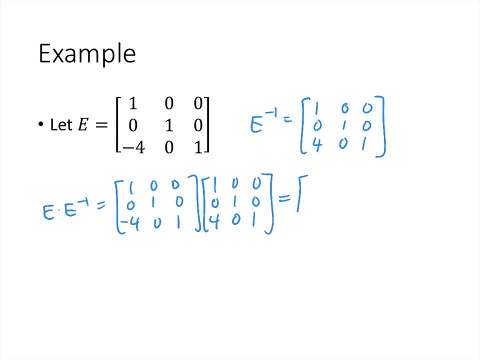 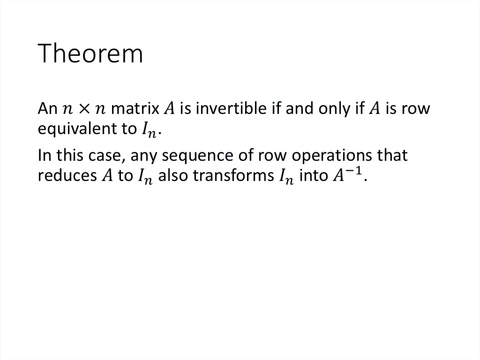 identity. And when we multiply this out, lo and behold, we do in fact get the identity matrix, with 1s down the diagonal and 0s everywhere else. Similarly, when we multiply in this order, again, we get the identity matrix. Okay, so what are all these elementary matrices? 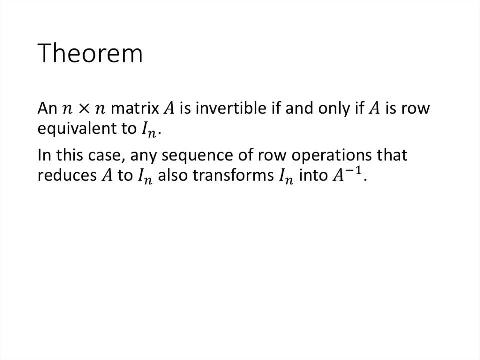 good for. Well, we have this theorem which is going to tell us exactly how to figure out, first of all, when a matrix is invertible and, in addition to that, how to actually figure out what the inverse of that matrix is. So the theorem says two. 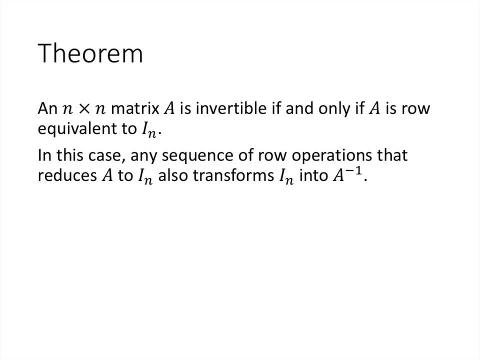 things. It says that a square matrix, A, is invertible if, and only if, A is row equivalent to the identity matrix. Remember, row equivalent here just means that it can be row-reduced into the identity matrix And any sequence of row operations that reduces A to the 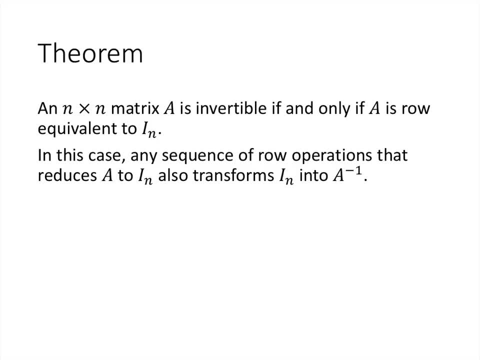 says that a square matrix, A, is invertible if, and only if, A is rho equivalent to the identity matrix. Remember, rho equivalent here just means that it can be rho reduced into the identity matrix, And any sequence of rho operations that reduces A to the identity matrix will turn out to. 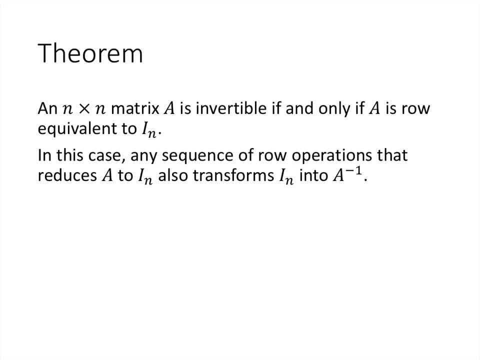 also transform the identity matrix into A inverse. So in other words, if we keep track of all of the different steps that we take, all of the different rho operations that we take to transform A into the identity matrix, and we perform those same steps in the same order, we will transform the 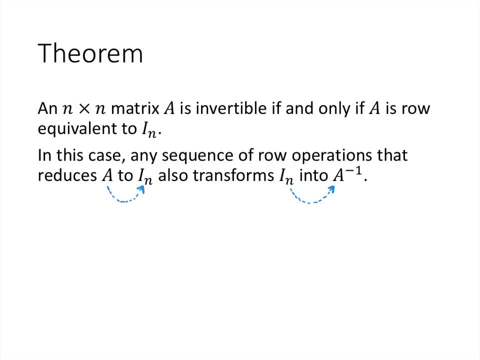 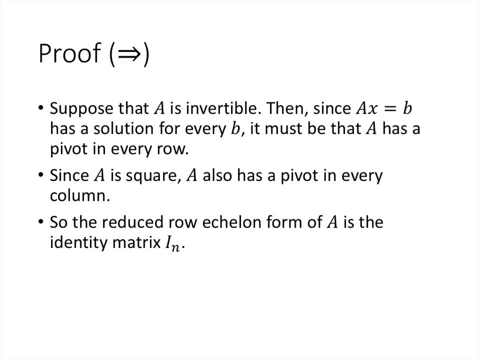 identity matrix into A inverse And we'll see how that turns out in the proof. Okay, Our theorem is an if and only if, which means we have to prove that the first statement implies the second statement and the second statement implies the first statement. The first statement. 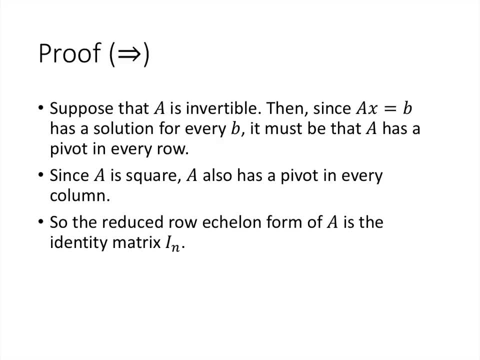 was that A was invertible, and the second statement was that A was rho equivalent to the identity matrix. So let's start by assuming that A is invertible. Now, we talked about that. this means that the matrix equation AX equals B has a solution for every B, and so it must be that capital A has. 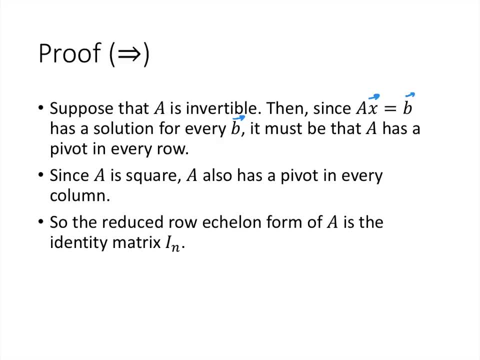 a pivot in every row, Because if capital A didn't have a pivot in every row, then that equation wouldn't be a pivot in every row. So we have to prove that the matrix equation AX equals B has a consistent for every possible vector B. That's something we talked about a while back. But A is a. 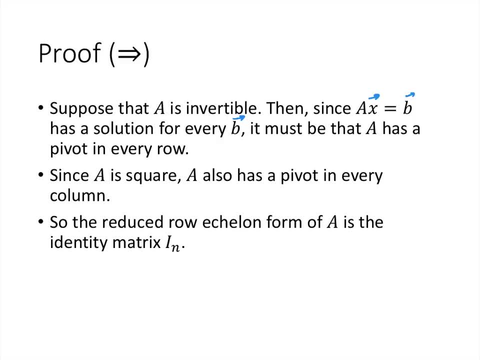 square matrix. So if it has a pivot in every row it's got to have a pivot in every column. And then the reduced row echelon form of that matrix, A. it's got a pivot in every row and a pivot every column. it's square. That's the identity matrix And that means that A is rho equivalent to the. 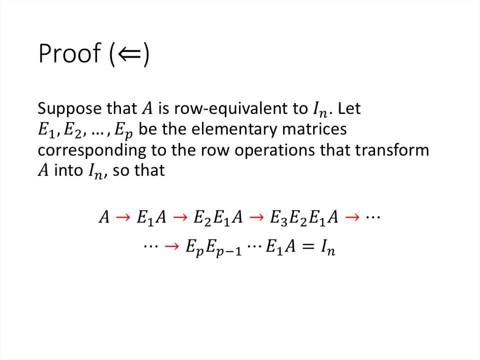 identity matrix. Now, going the other direction is where the elementary matrices are going to come in. So we're going to suppose that A is rho, equivalent to the identity matrix. So that means that there's some sequence of steps, each one a single row operation, And when we do, 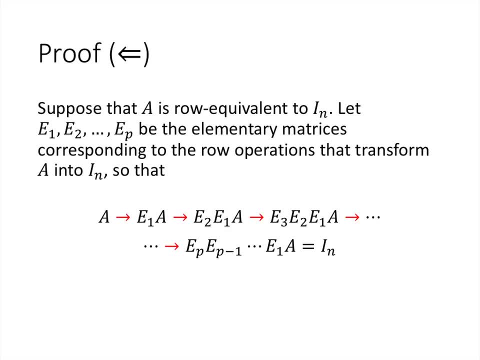 those steps in order: we start with A and we end up with the identity matrix. So let's actually write down what those steps are And each one of them can be represented by an elementary matrix. So E1, that's the first step, the first row operation that we need to turn A into the identity. 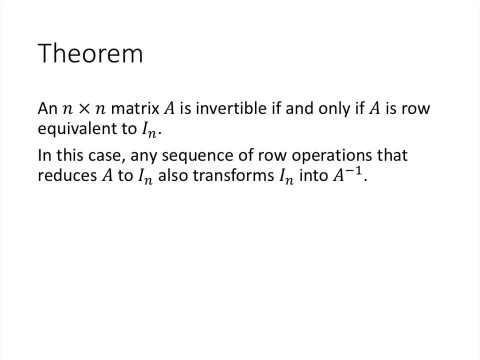 identity matrix will turn out to also transform the identity matrix into A inverse. So, in other words, if we keep track of all of the different steps that we take, all of the different row operations that we take to transform A into the identity matrix, 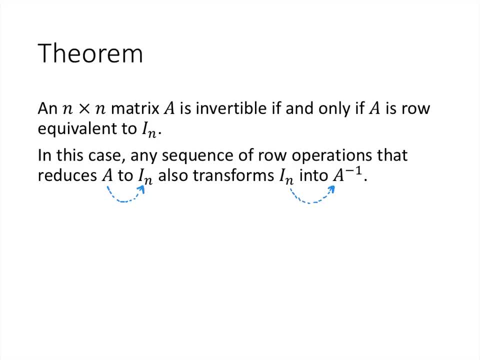 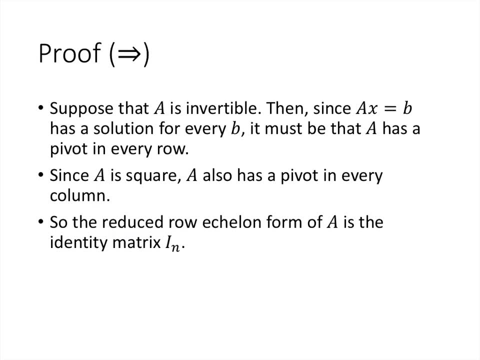 and we perform those same steps in the same order, we will transform the identity matrix into A inverse And we'll see how that turns out in the proof. Okay, our theorem is an if and only if, which means we have to prove that the first statement implies the second statement. 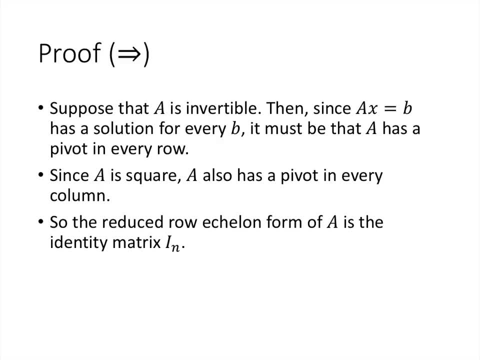 and the second statement implies the first statement. The first statement was that A was invertible and the second statement was that A was row equivalent to the identity matrix. So let's start by assuming that A is invertible. Now we talked about that. this means that the matrix equation- 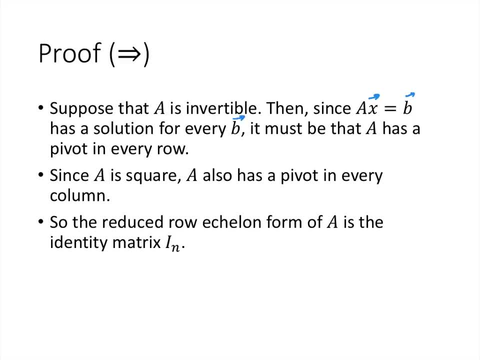 AX equals B has a solution for every B, and so it must be that capital A has a pivot in every row, Because if capital A didn't have a pivot in every row, then that equation wouldn't be consistent for every possible vector B. 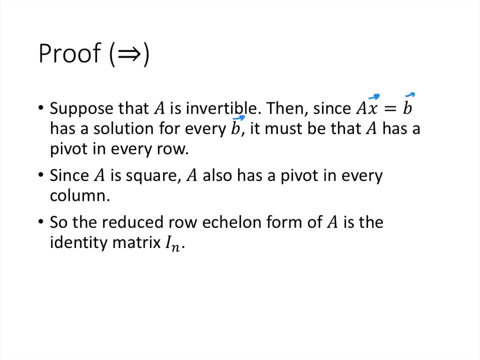 That's something we talked about a while back. But A is a square matrix, So if it has a pivot in every row, it's got to have a pivot in every column And then the reduced row echelon form of that matrix, A. 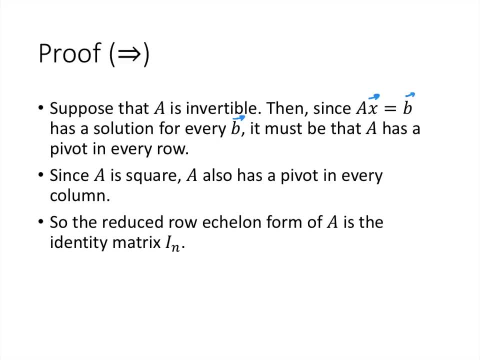 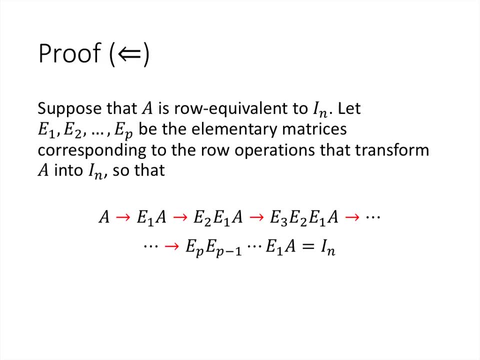 it's got a pivot in every row and a pivot in every column. it's square, That's the identity matrix And that means that A is row equivalent to the identity matrix. Now, going the other direction is where the elementary matrices are going to come in. 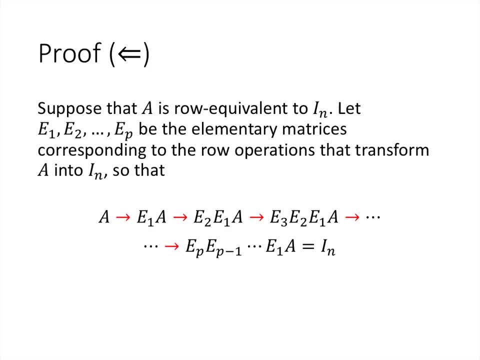 So we're going to suppose that A is row equivalent to the identity matrix. So that means that there's some sequence of steps, each one a single row operation, And when we do those steps in order, we start with A and we end up with the identity matrix. 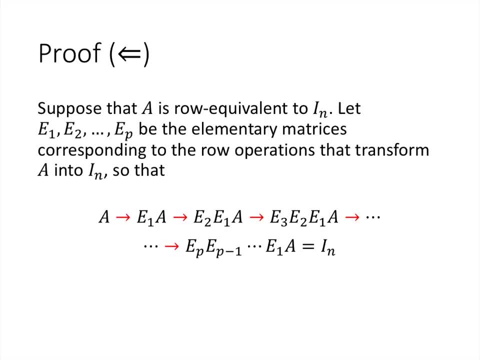 So let's actually write down what those steps are, And each one of them can be represented by an elementary matrix. So E1, that's the first step, the first row operation that we need to turn A into the identity matrix, And E2, that's the matrix. 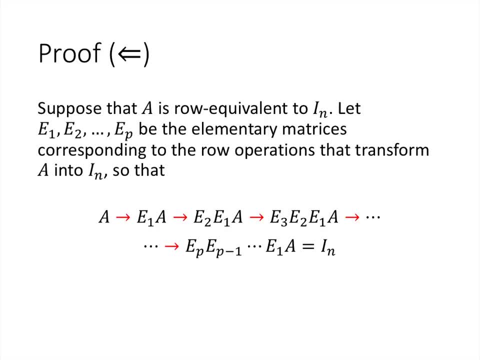 the elementary matrix. that represents the second step in transforming A into the identity matrix, And so on and so on, And however many steps it takes, we're going to say it takes P steps here. So that number P is just if it takes 533 steps. 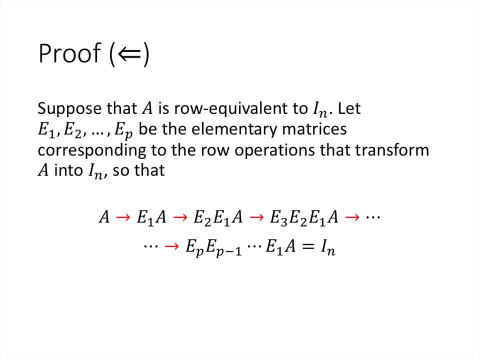 matrix And E2, that's the matrix, the elementary matrix, that represents the second step in transforming A into the identity matrix, And so on and so on. And however many steps it takes, we're going to say it takes P steps here. 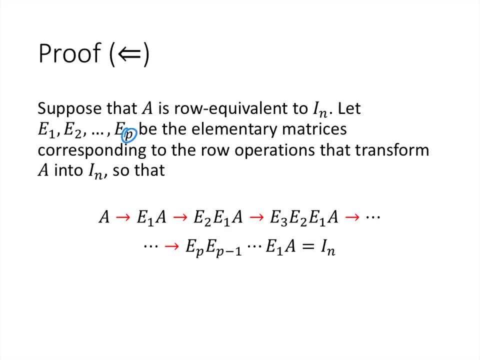 So that number P is just. if it takes 533 steps, then that's what P is. If it takes four steps, then P is four, however many steps it takes. But remember that we can represent the result of doing one of those steps by multiplying by an elementary matrix. So the first step here is we multiplied by 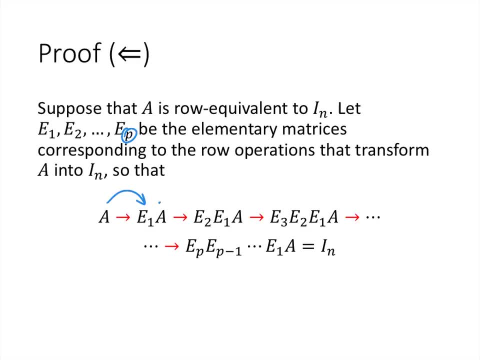 the matrix E1. And then the second step is we take the result and multiply it by E2.. So now we've multiplied by two elementary matrices. And so that's the first step. And then the second step is we take the result and multiply it by E2.. 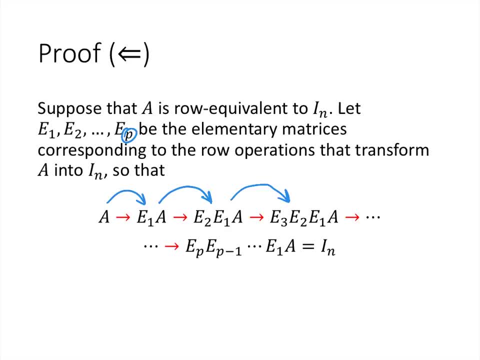 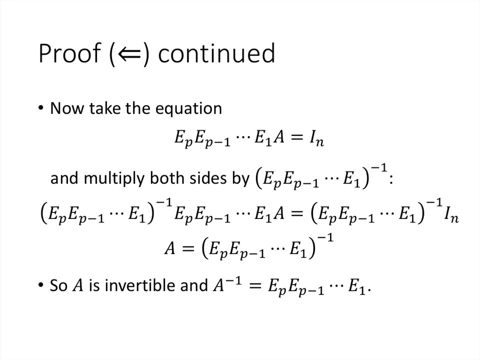 And now we're going to multiply by three elementary matrices, And so on and so on, until we've multiplied by all of the elementary matrices And the result is the identity. So this equation is going to be the equation that's going to work for us. So we're going to take that equation and 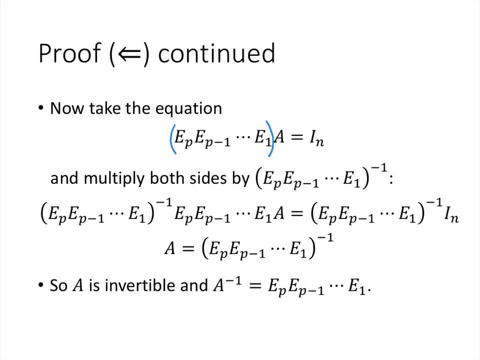 multiply both sides by the inverse of the product of all of the elementary matrices. So on the left hand side we've multiplied by an inverse, multiplied by the same matrix, And so we're going to multiply by the matrix. So those are going to cancel out. So on the left hand side we just get A, And on the right hand 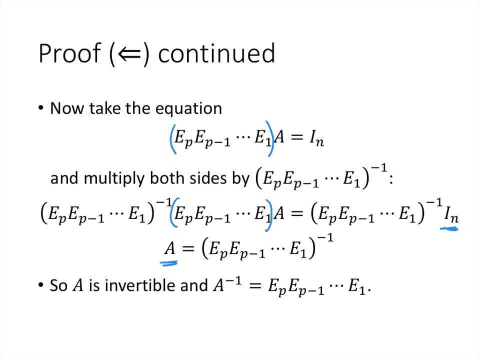 side we multiplied by the identity, And multiplying by that, multiplying by the identity, doesn't do anything, And so we get that A is the inverse of all of those elementary matrices. But that means that we can take the inverse of both sides And we just get that A inverse is the product of all. 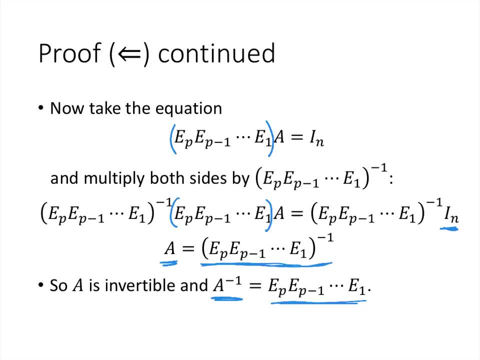 those elementary matrices. And if we tack on a little identity matrix here, then multiply by the identity matrix, by all of those elementary matrices. that shows us the second part of what the theorem says, which is that the inverse of A is the result of applying all of those elementary 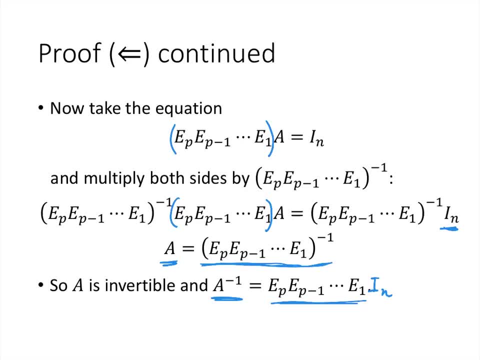 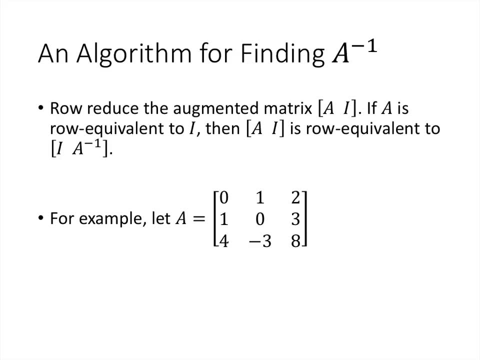 row operations to the identity matrix. Now, if we take the theorem at base value, what it sounds like we're going to have to do is keep track of every single step we take in row reducing the matrix, and keep track of what all those steps are and then recreate those steps on the identity. 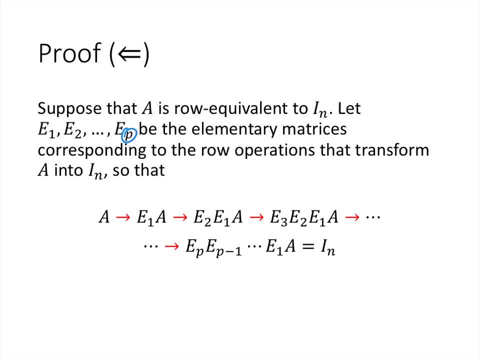 then that's what P is. If it takes four steps, then P is four, However many steps it takes. But remember that we can represent the result of doing one of those steps by multiplying by an elementary matrix. So the first step here is we multiply by the matrix at E1. 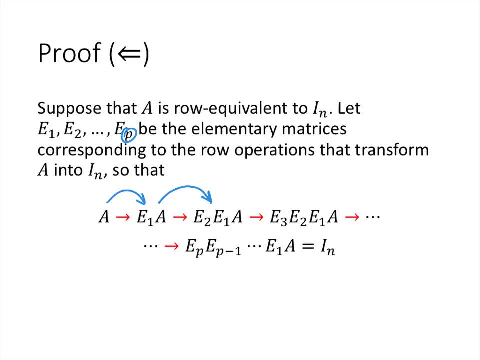 And the second step is we take the result and multiply it by E2.. So now we have multiplied by two elementary matrices, And now we are going to multiply by three elementary matrices, And so on, and so on, until we've multiplied by all of the elementary matrices and the result is the identity. 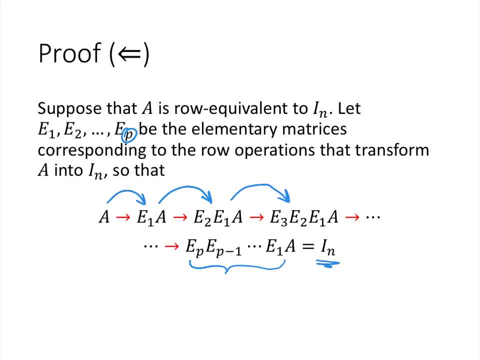 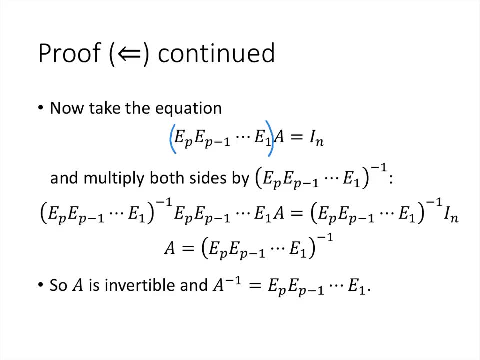 So this equation is going to be the equation that's going to work for us. So we're going to take that equation and multiply both sides by the inverse of the product of all of the elementary matrices. So on the left-hand side we've multiplied by an inverse multiplied. 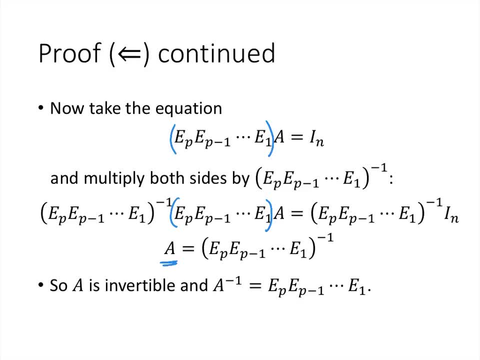 by the same matrix. so those are going to cancel out. So on the left-hand side we just get a, and on the right-hand side we multiplied by the identity, and multiplying by the identity doesn't do anything, and so we get that. a is the inverse of all of those elementary matrices. 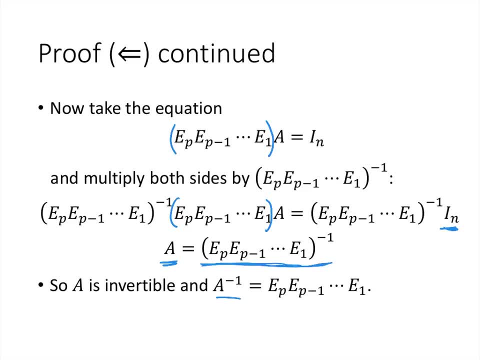 But that means that we can take the inverse of both sides and we just get that a inverse is the product of all those elementary matrices And if we tack on a little identity matrix here, then multiplying the identity matrix by all of those elementary matrices, 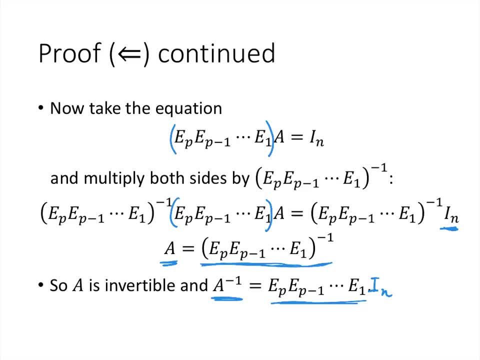 that shows us the second part of what the theorem says, which is that the inverse of a is the result of applying all of those elementary row operations to the identity matrix. Now, if we take the theorem at base value, what it sounds like we're going to have to do is keep. 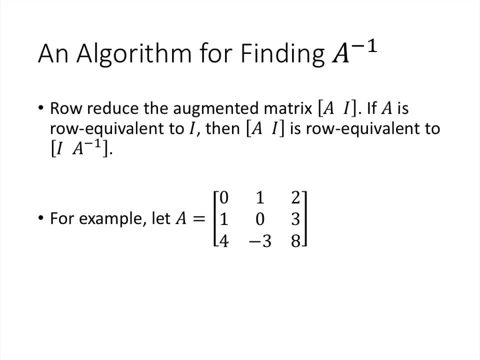 track of every single step we take in row, reducing the matrix, and keep track of what all those steps are and then recreate those steps on the identity matrix. But it turns out we don't have to work that hard because what we can do is basically: 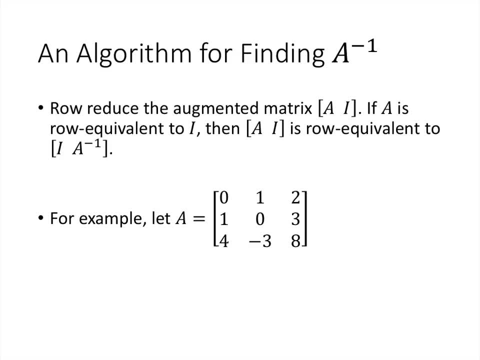 row reduce a double matrix. So we're going to augment our matrix a with a copy of the identity matrix. So we're going to take our matrix a, which in this case is 0, 1, 2, 1, 0, 3,, 4, negative 3,. 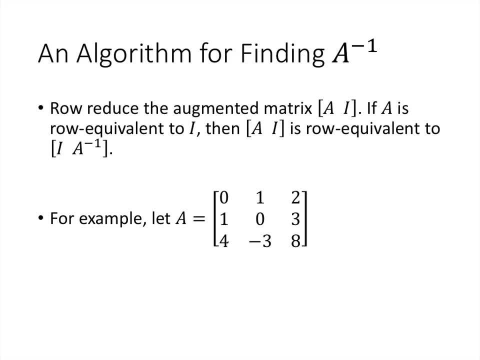 matrix. But it turns out we don't have to work on that. We don't have to work on the identity matrix, Because what we can do is basically row, reduce a double matrix. So we're going to augment our matrix A with a copy of the identity matrix. So we're going to take our matrix A, which, in this, 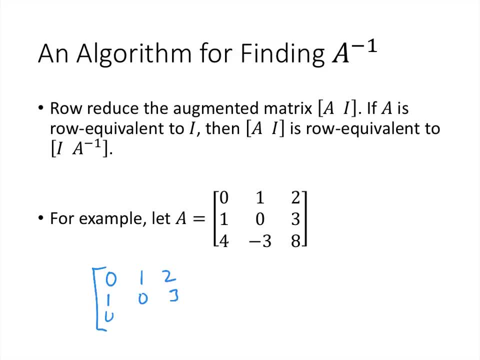 case is 0, 1, 2, 1, 0, 3, 4, negative 3, 8.. And we're going to tack onto it a copy of the identity matrix And this double matrix so you can imagine there's sort of like a imaginary dotted line. 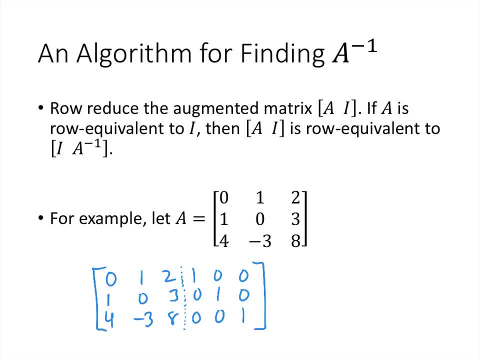 there. That double matrix is going to be a copy of the identity matrix, And so we're going to row reduce that And eventually, what this is going to turn out to be is, because A is invertible, A is going to get row reduced into the identity matrix, And the 4th, 5th and 6th 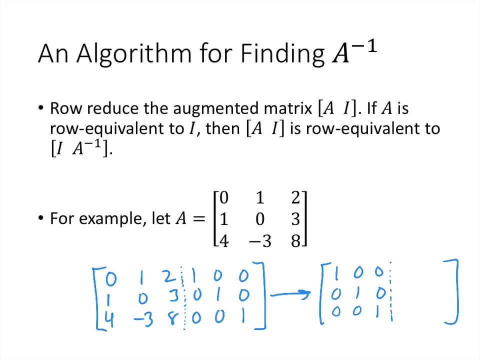 columns here are just going to get carried along for the ride. And so what's going to be here once we're done row reducing? That's going to be A inverse, Because we're going to have performed the same row operations to that second half of that matrix. All right, let's see this in action. 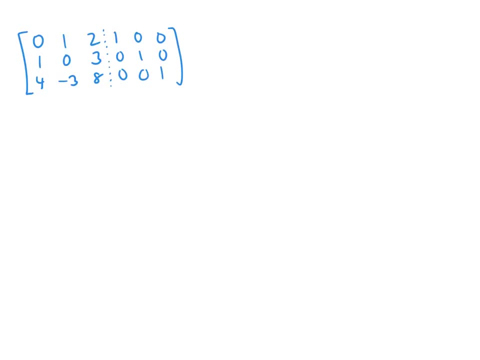 Okay. so if we want to reduce this matrix, first thing we need to do is get a pivot in the first row, first column. So we're going to swap rows 1 and 2.. So now row 1 is 1, 0, 3, 0, 1, 0, 0, 1, 2,. 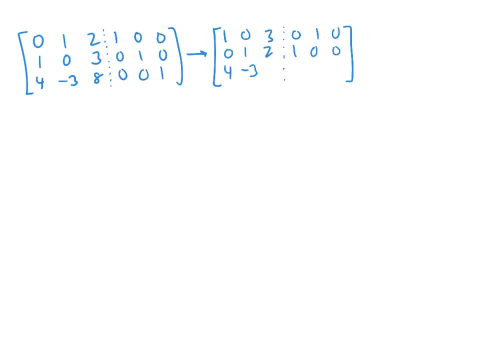 1,, 0,, 0, and 4, negative 3, 8,, 0,, 0,, 1.. Now we need zeros below that first pivot. So we're going to multiply row 1 by negative 4. And we're going to get a pivot in the first row, first column. 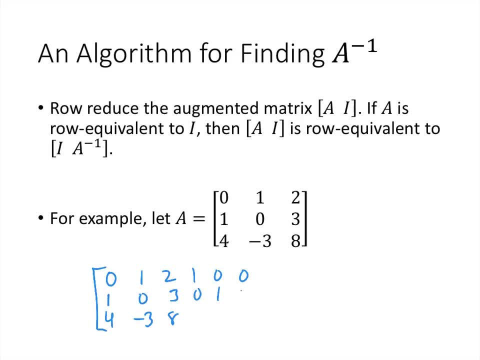 8, and we're going to tack onto it a copy of the identity matrix And this double matrix, so you can imagine there's sort of like a imaginary dotted line there, that double matrix. we're going to row, reduce that And eventually what this is going to turn out to be is because a is invertible. 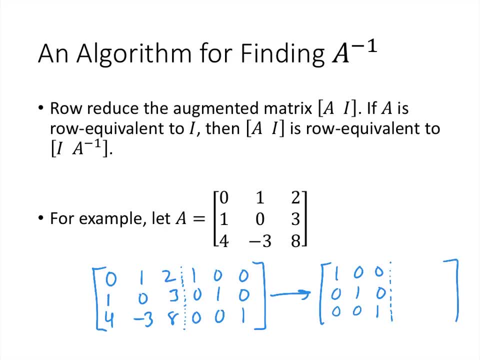 a is going to get row reduced into the identity matrix, And the fourth, fifth and sixth columns here are just going to get carried along for the ride. And so what's going to be here once we're done row reducing? That's going to be a inverse. 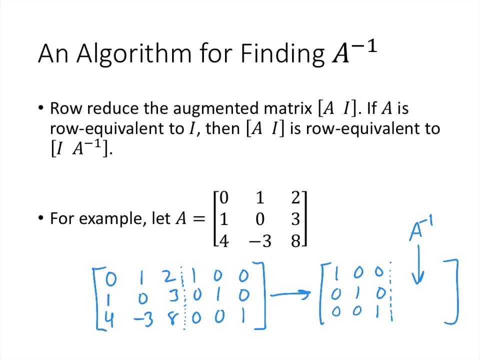 because we're going to have performed the same row operations to that second half of that matrix. All right, let's see this in action. Okay, so if we want to row reduce this, we're going to have to do a row reduction. 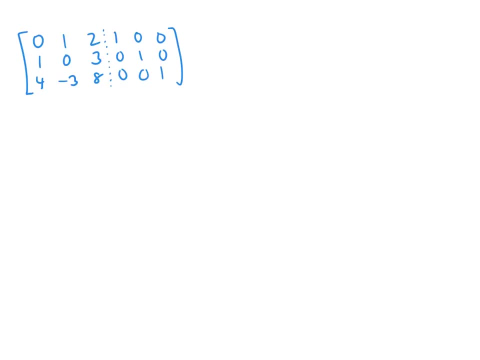 First thing we need to do is get a pivot in the first row, first column. So we're going to swap rows 1 and 2.. So now row 1 is 1, 0, 3, 0, 1, 0, 0, 1, 2, 1, 0, 0, and 4, negative: 3, 8, 0, 0, 1.. 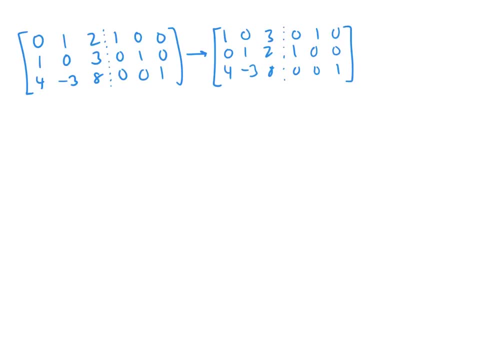 Now we need zeros below that first pivot. so we're going to multiply row 1 by negative 4 and add the result to row 3.. So that's not going to change row 1.. It's not going to change row 2.. 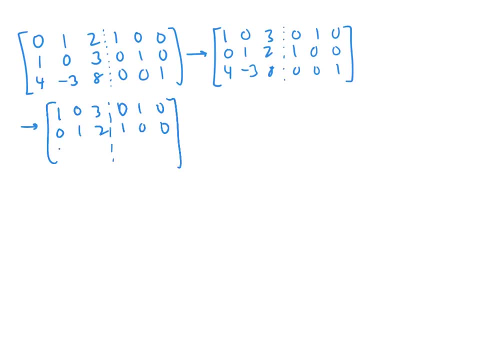 It is going to change row 3.. So multiplying by negative 4, that gives us a 0 there, We're still going to have a negative 3 there. Negative 4 times 3 is negative 12, plus 8 is negative 4.. 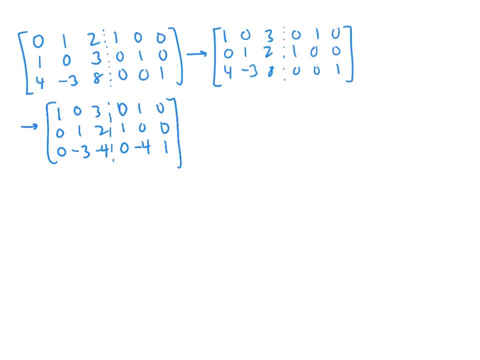 That's still going to be a 0.. We get a negative 4 and a 1.. Now in the second column we have a 1 where we want it, so that's good. We need to get rid of that negative 3.. 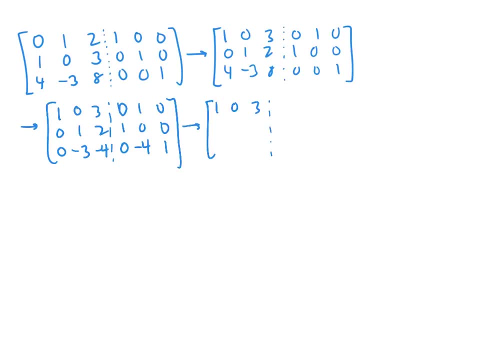 So row 1 is OK for now, leaving row 2 alone, and then row 3 is going to change again. So we're multiplying row 2 by positive 3 and adding it to row 3.. That gives us a 0 there. 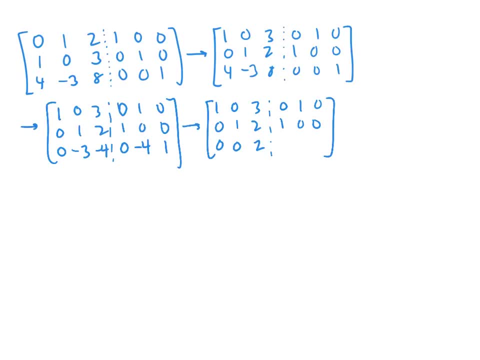 2 times 3 is 6, plus negative 4 is 2.. 3 times 1 is 3.. Add to 0, gives me 3.. And then this will still be a negative 4 and a 1.. 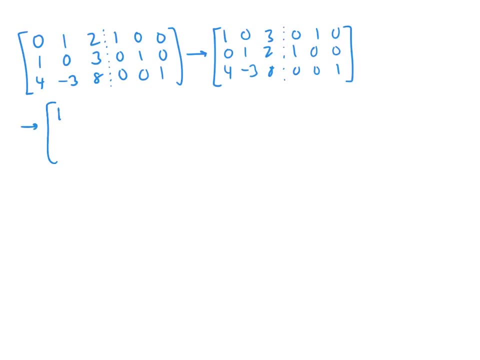 And add the result to row 3.. So that's not going to change row 1.. It's not going to change row 2.. It is going to change row 3.. So multiplying by negative 4, that gives us a 0. there We're still. 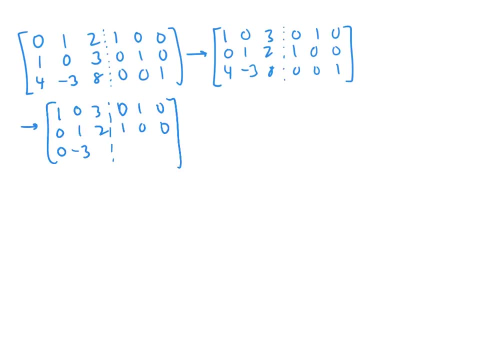 going to have a negative 3 there. Negative 4 times 3 is negative 12, plus 8 is negative 4.. That's still going to be a 0. We get a negative 4 and a 1.. Now in the second column we have a 1. And we're going to get a 1. And we're going to get a 1.. 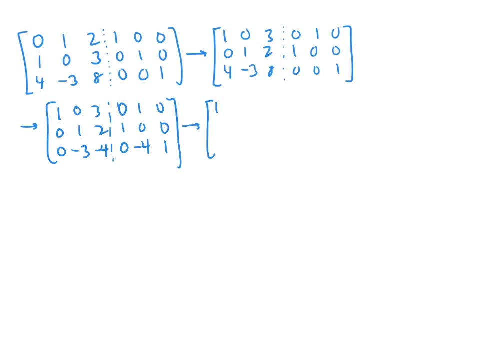 We need to get rid of that negative 3.. So row 1 is OK for now, Leaving row 2 alone, And then row 3 is going to change again. So we're multiplying row 2 by positive 3 and adding it to row 3.. That gives 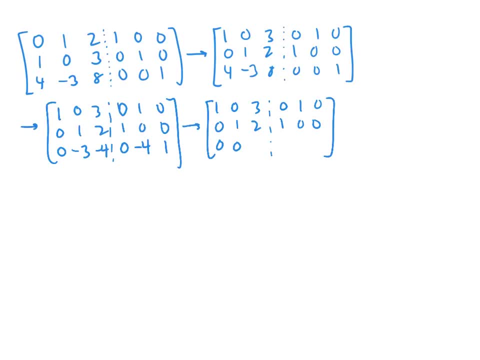 us a 0 there. 2 times 3 is 6, plus negative 4 is 2.. 3 times 1 is 3.. That to 0 gives me 3.. And then this will still be a negative 4 and a 1.. 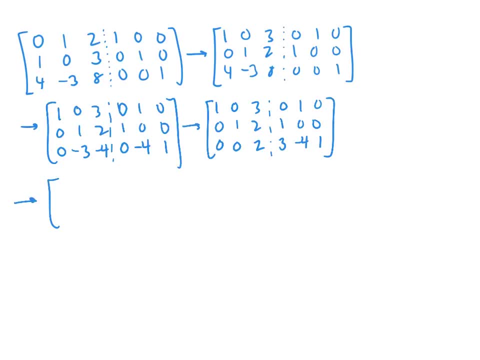 Now, finally, we have to fix the third column. So first thing we'll do is we'll divide row 3 by 2.. That's going to give us 3 halves, Negative 2 and 1 half, And then we need to get rid of the 3 and 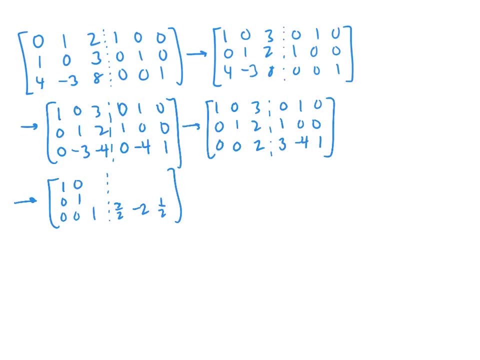 the 2 above that. So we're going to multiply row 3 by negative 3 and add it to row 1.. That gives me a 0.. Negative 3 times 3 halves is negative 9.. And then we're going to divide row 3 by negative 3.. That 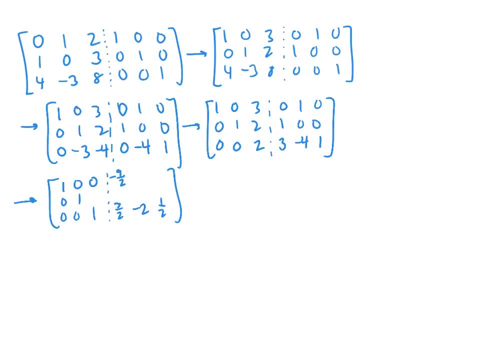 will give us negative 9 halves plus 0. That's negative 9 halves Negative. 3 times negative. 2 is positive 6, plus 1 is 7.. And then negative 3 times a half is negative. 3 halves plus 0 is negative 3. 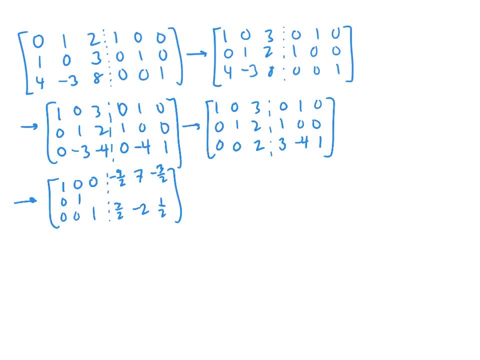 halves. And then we need to multiply row 3 by negative 2 and add it to row 2.. That will give me a 0 there. Negative 2 times 3: halves is negative 3, plus 1 is negative 2.. Negative 2 times negative 2. 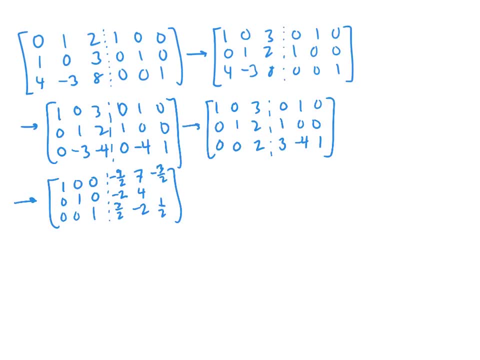 is positive, 4, plus 0 is positive 4. And negative: 2 times 1. half is negative. 1, plus 0 is negative 1.. So we've successfully gotten the identity matrix here, And so what we have here in the second half. 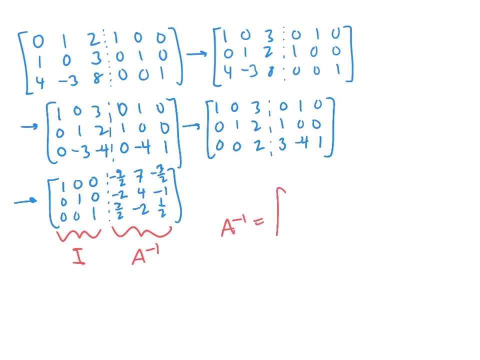 of the matrix that turns out to be a inverse. So a inverse is the matrix: Negative: 9 halves 7, negative: 3 halves negative 2, 4, negative 1, 3 halves negative 2, 1 half. 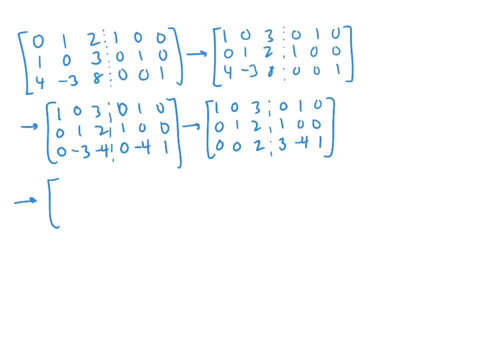 Now, finally, we have to fix the third column. So first thing we'll do is we'll divide row 3 by 2.. That's going to give us 3 halves negative 2 and 1 half, And then we need to get rid of the 3 and the 2 above that. 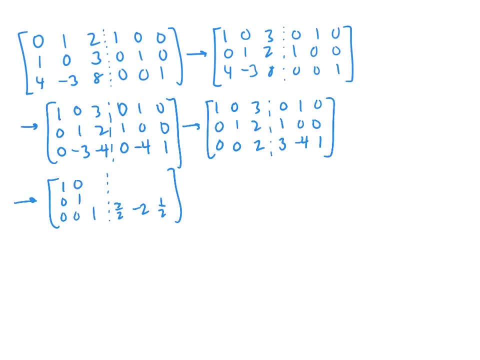 So we're going to multiply row 3 by negative 3 and add it to row 1.. That gives me a 0.. Negative 3 times 3 halves is negative 9 halves plus 0.. That's negative 9 halves. 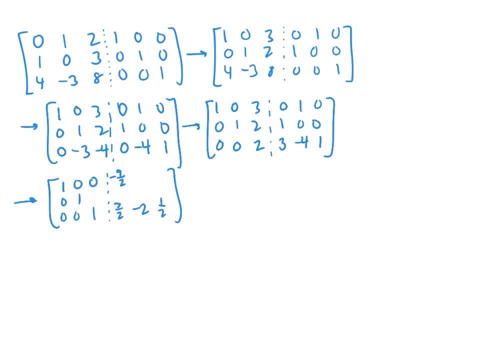 Negative 3 times negative 2 is positive 6, plus 1 is 7.. And then negative 3 times a half is negative 3 halves plus 0 is negative 3 halves. And then we need to multiply row 3 by negative 2 and add it to row 2.. 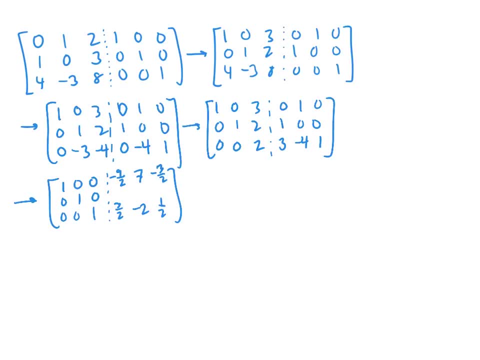 That will give me a 0 there. Negative 2 times 3 halves is negative. 3, plus 1 is negative 2. Negative 2 times negative: 2 is positive. 4, plus 0 is positive, 4.. And negative 2 times 1: half is negative. 1, plus 0 is negative 1.. 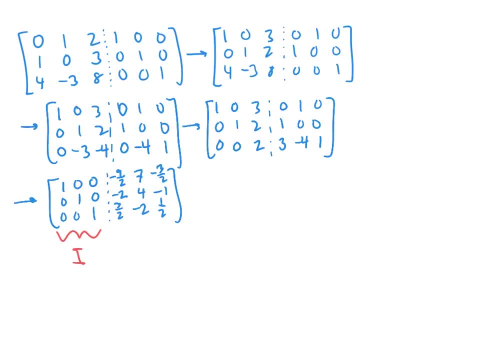 So we've successfully gotten the identity matrix here And so what we have here in the second half of the matrix that turns out to be A inverse. So A inverse is the matrix: negative 9 halves 7, negative 3 halves negative 2, 4, negative 1,. 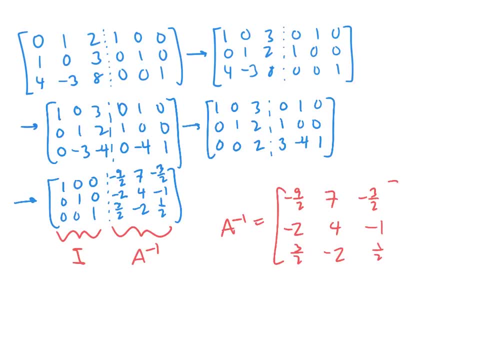 3 halves negative 2, 1 half, And we can verify that by multiplying row 3 by 2.. And we can verify that by multiplying this by the original matrix A on both sides, to make sure that we get the identity matrix. 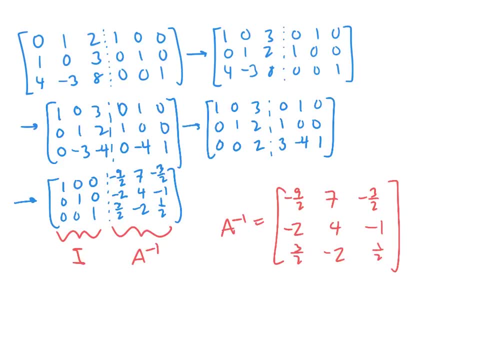 But if we believe the proof of the theorem, then this is exactly what we would get if we did all of those row operations to the identity matrix, Because that's exactly what we did At every step. every time we did a row operation, we were doing the row operations to all of these columns number 4, 5, and 6.. 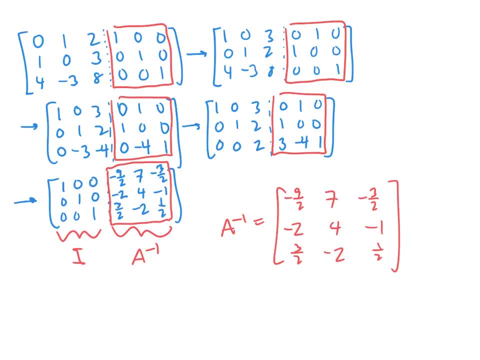 We were doing the row operations to that second half of that matrix And this process would work for 4 by 4 matrices, 5 by 5 matrices, 6 by 6 matrices. Obviously, the bigger the matrix gets, the more steps it would take. 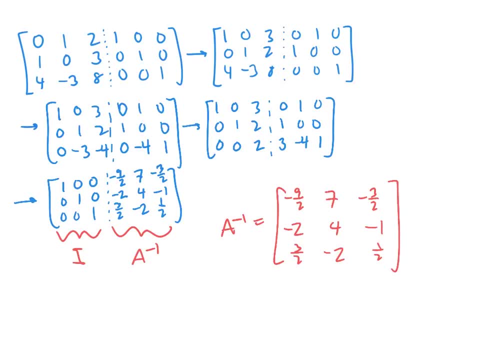 And we can verify that by multiplying this by the original matrix A on both sides, to make sure that we get the identity matrix. But if we believe the proof of the theorem, then this is exactly what we would get if we did all of those row operations to the identity matrix, Because that's exactly what. 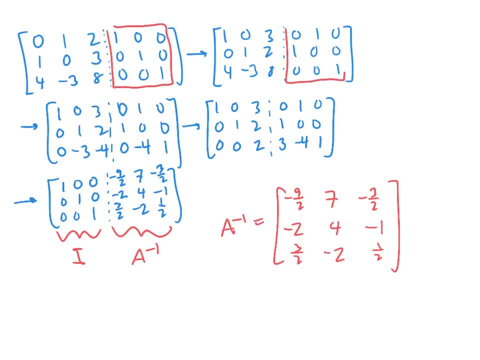 we did At every step, every time we did a row operation. we were doing the row operations to all of these four, the columns number 4, 5, and 6. We were doing the row operations to that second half of that matrix. 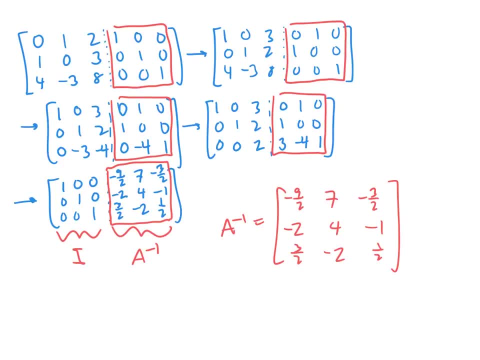 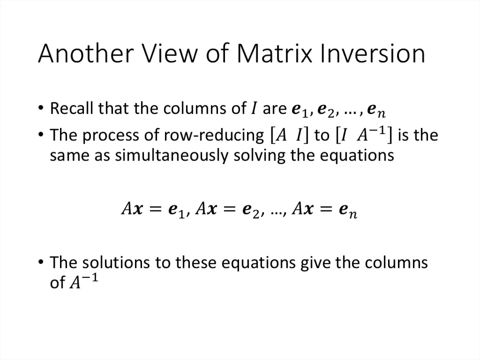 The general process would work for 4x4 matrices, 5x5 matrices, 6x6 matrices. Obviously, the bigger the matrix gets, the more steps it would take, But the general process works. Now, another way that we can look at what we're doing here is that, if we remember that the columns 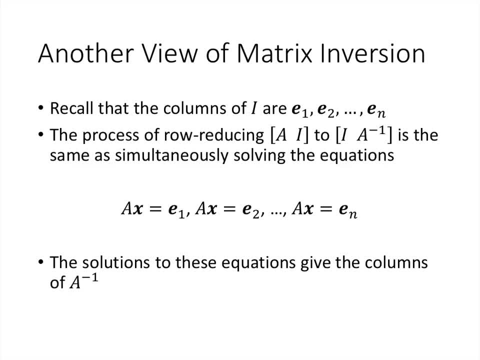 of the identity matrix are these standard basis vectors E1, E2, and so on. then the process of row reducing the double matrix AI to I A inverse- is the same as simultaneously solving the equations AX equals E1,, AX equals E2, and so on, Because for that we have an augmented 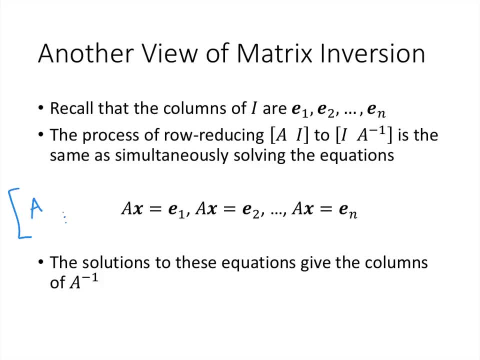 matrix, where the augmented matrix looks like capital A here, and then we only have one additional column where we have some standard basis vector there. But again the idea is all of the row operations are really happening over here and the vector EI is just getting carried. 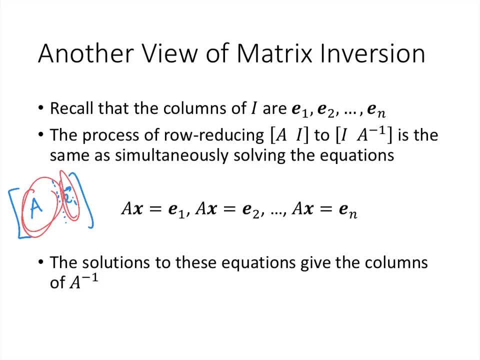 along for the ride. So we're just doing that n times, We're solving n systems of equations simultaneously, And the solutions in each of those additional, extra augmented columns gives us a column of A inverse. 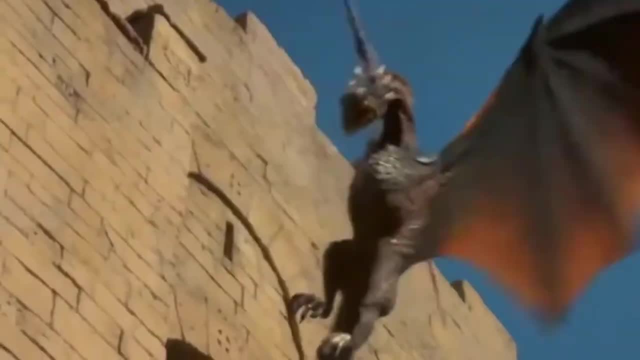 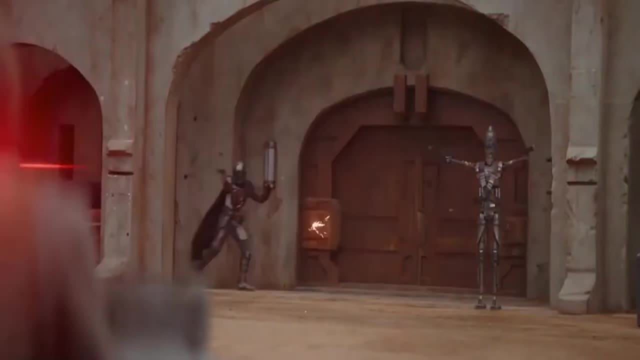 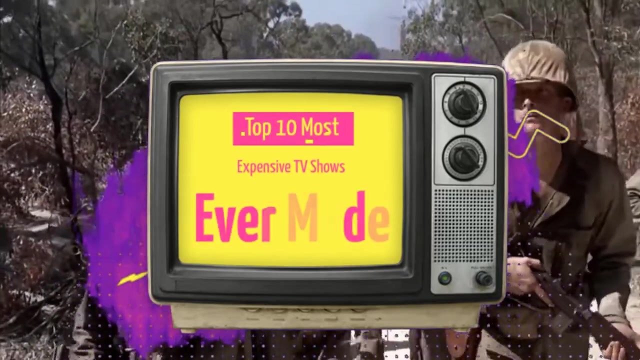 It's no wonder that television series have grown in popularity. The market for internet media streaming is becoming increasingly competitive by the minute. Companies are investing millions of dollars in the creation of high-quality shows. today, Here are the top 10 most expensive TV shows ever made so far. But before we get started, be sure to subscribe to our channel and ring the bell to get notified about our latest videos. Number 10, The Morning Show: $15 million per episode When Apple TV Plus launched, alongside its flagship show, The Morning Show in 2019,. 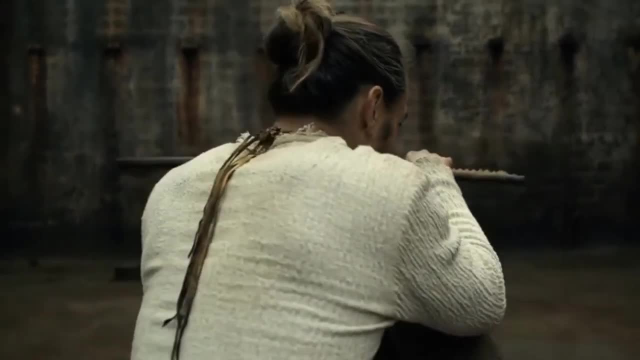 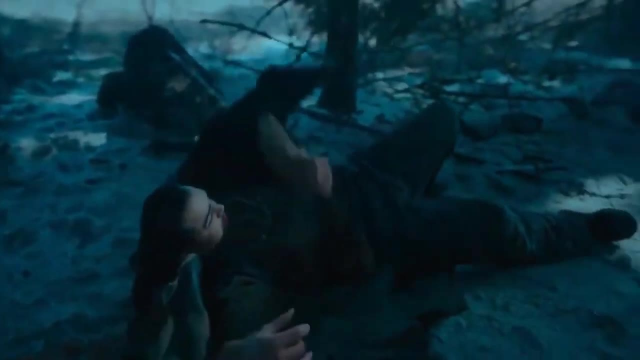 The Apple TV Plus series See, set in a dystopian future where humanity has lost the capacity to see, chronicles the narrative of the impact of the birth of two children who are capable of seeing in a world where this gift is deemed heresy.